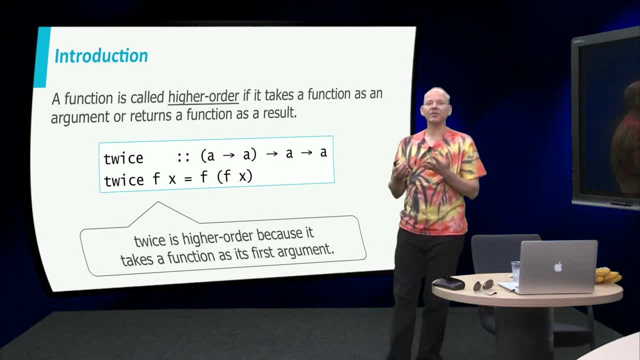 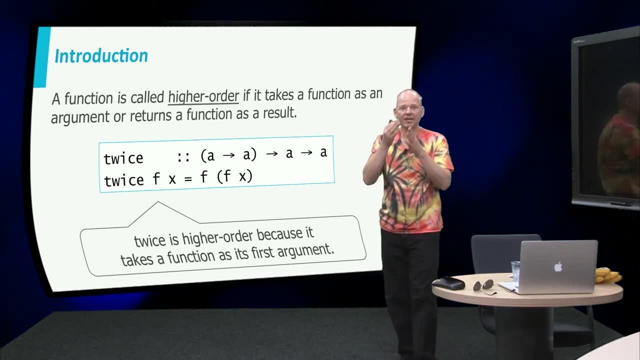 then on the right, we see that it takes as the first parameter a function from a to a and it returns a function from a to a And if we look at the definition again with that type in mind, we see that that type makes sense. 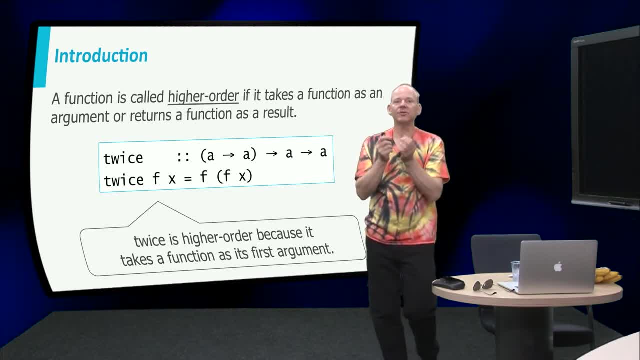 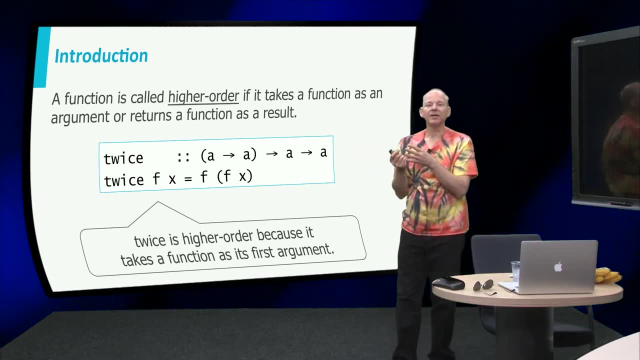 Twice takes a function. that function goes from A to A. then it takes an argument of type A, that's X, and then it returns a value of type A. Well, how does it do that? It applies F once which takes an A, transforms that into another A. 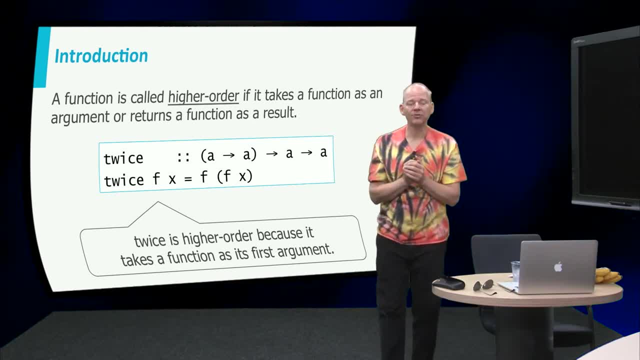 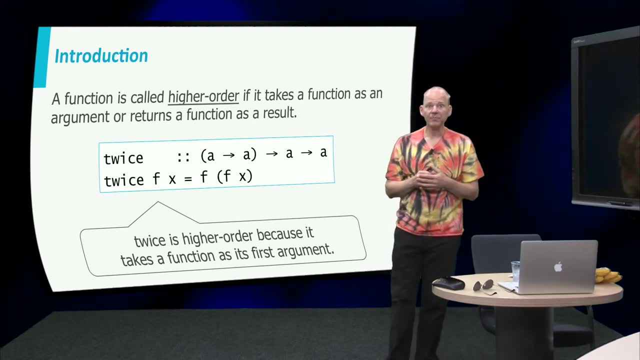 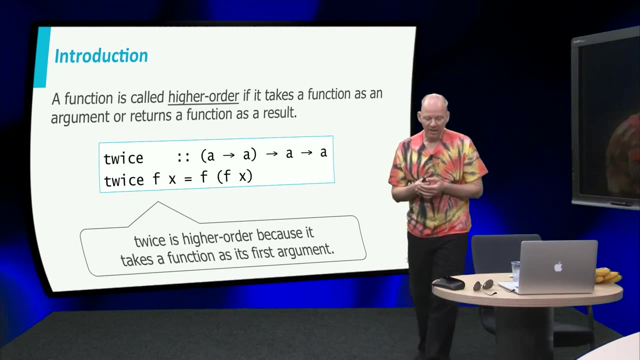 so the argument to the second application of F will also be of type A and you apply F a second time to return a value of type A. So twice is a higher order function because it takes a function as its first argument. Also, notice how the parentheses are used. 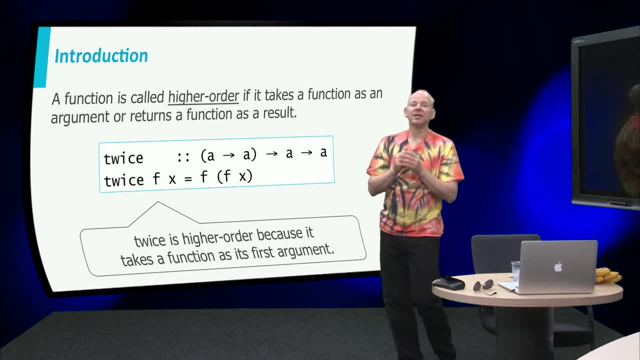 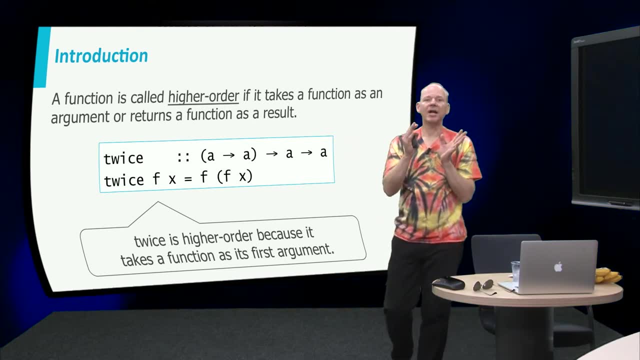 The parentheses on the first argument are explicit, because it's a function from A to A and the brackets for function types associate to the right, so we have to put the parentheses there, but we don't have to put them on the right-hand side. 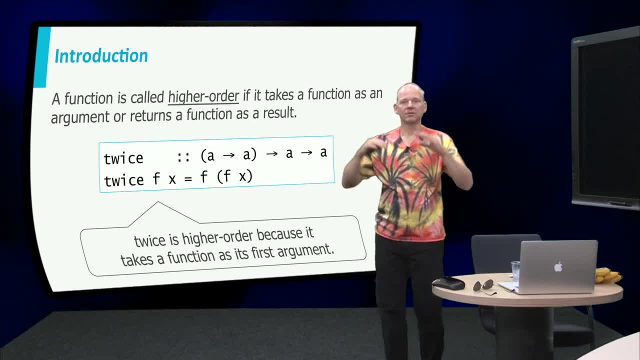 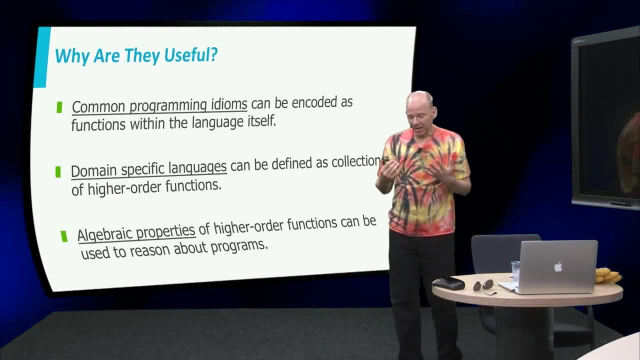 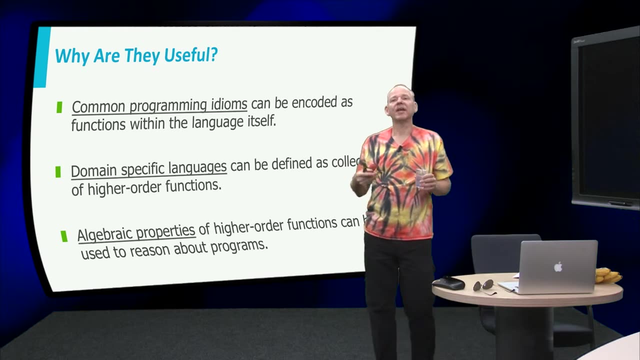 But if we would put all the parentheses, the type would look: A arrow, A arrow, A arrow A. Why are higher order functions useful? Well, there's this thing that programmers love to do, and that's not repeat yourself. Don't repeat yourself. 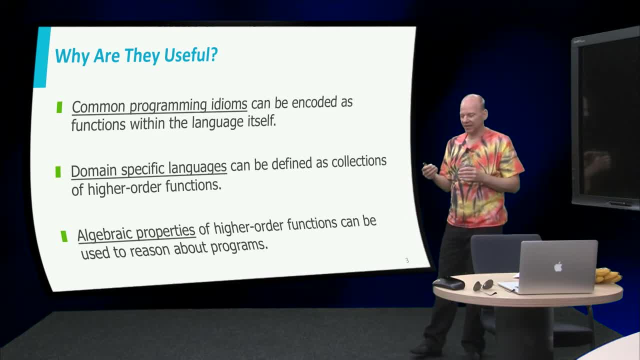 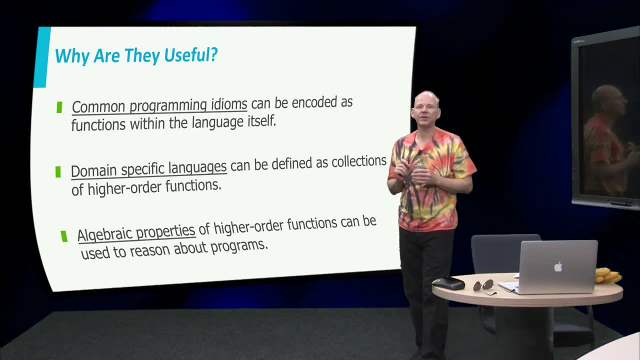 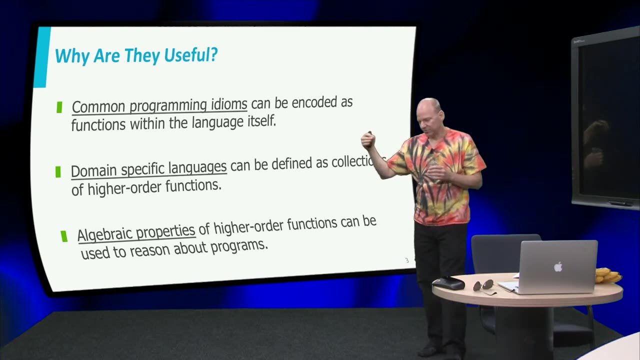 And with higher order functions we allow this thing to be encoded in the language, because whenever we see repetition we abstract that pattern into higher order functions and then we can apply that higher order function with various arguments to specify what is different between all the common uses of this common pattern. 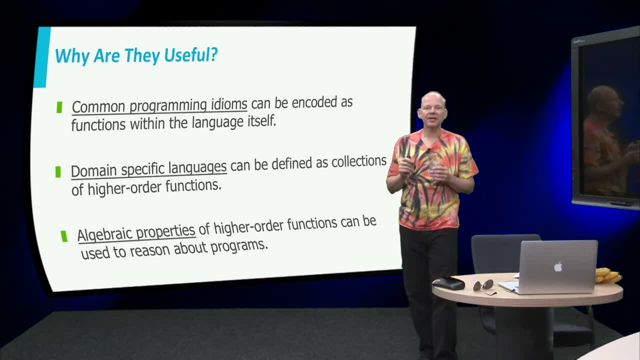 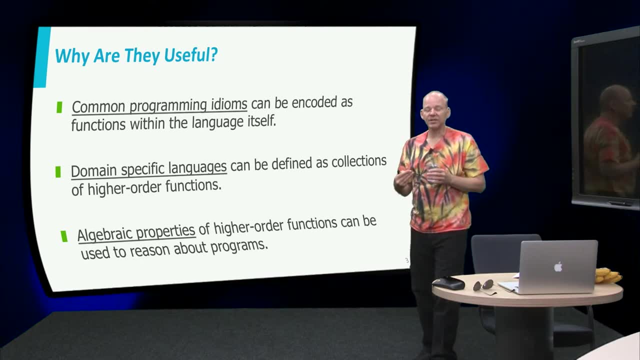 Okay, so common programming idioms can be encoded as functions within the language itself. And laziness here plays an important role, because if you don't have lazy evaluation, arguments might be evaluated prematurely. and then the evaluation, and then the evaluation. 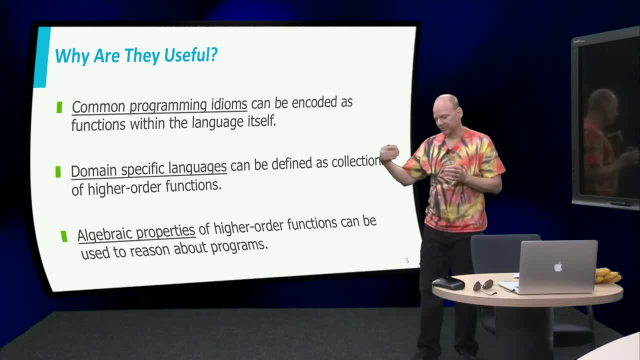 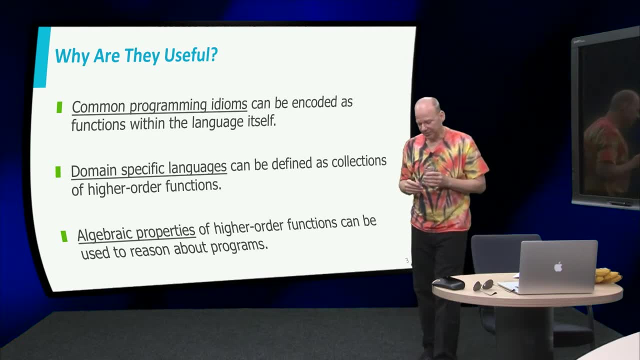 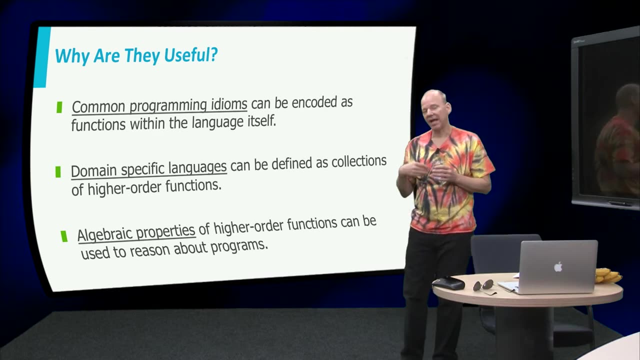 the effect is not the same as the pattern where you instantiate the arguments for the parameters. Another way to look at this is that we can define domain-specific languages as collection of higher order functions. So in Haskell people often talk about domain-specific languages where they mean APIs. 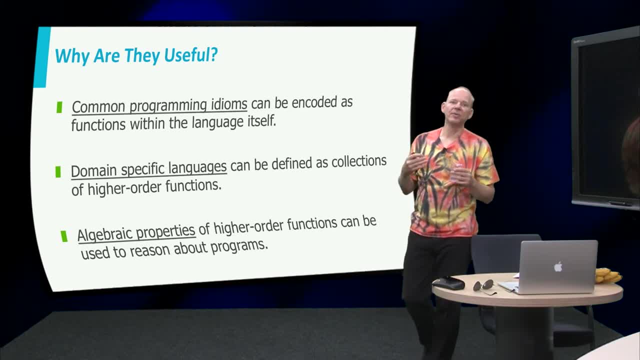 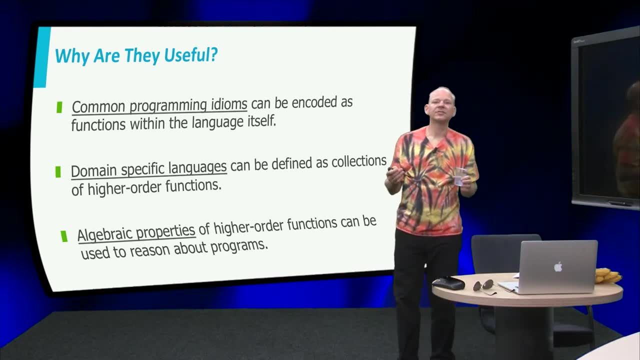 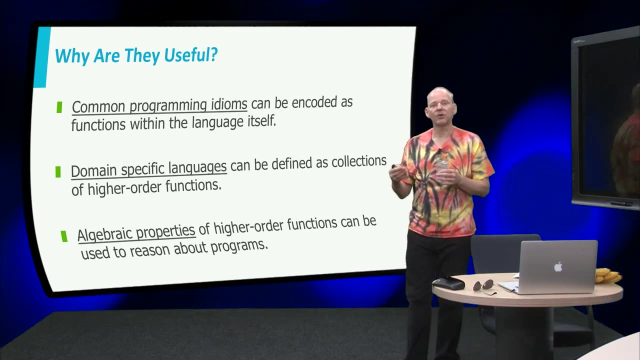 Okay, another way to say that is, these are embedded domain-specific languages. And then the third advantage of higher order functions is that these higher order functions have algebraic properties that we can use to reason about programs. And these higher order properties, these properties of higher order functions, 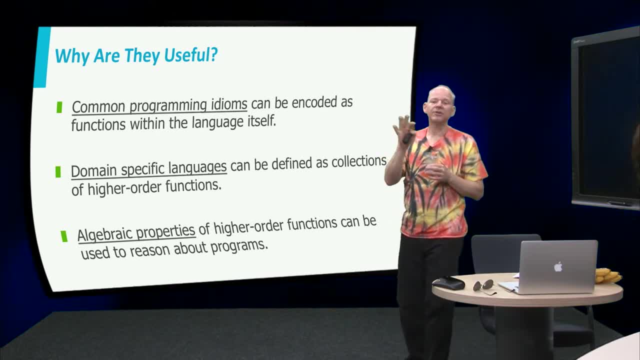 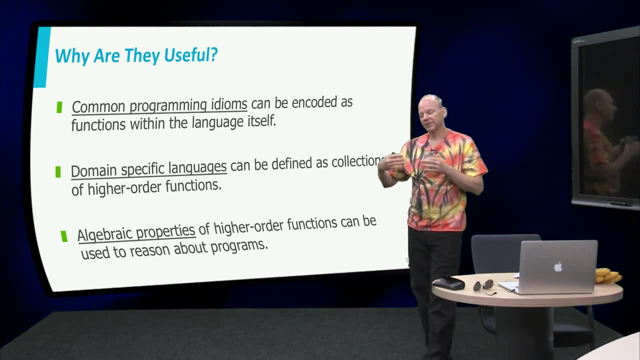 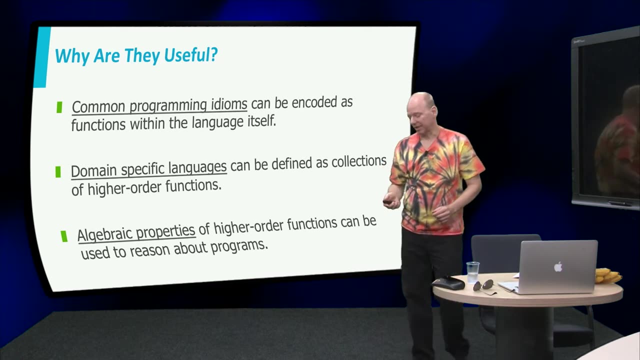 sorry, these algebraic properties they hold, irrespective of how you, which parameters you pass to them, So you can define properties of these programs, kind of in a general way, and then use, and then use them all along, And we will see several of these examples as we go. 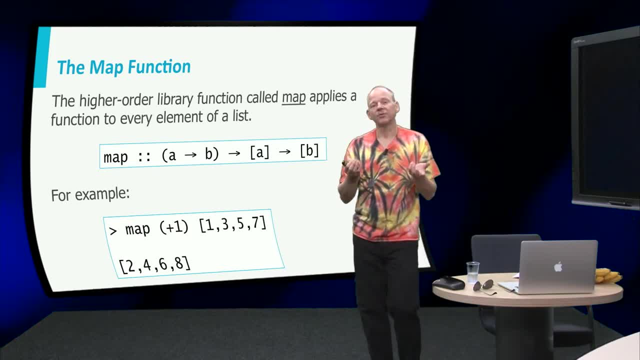 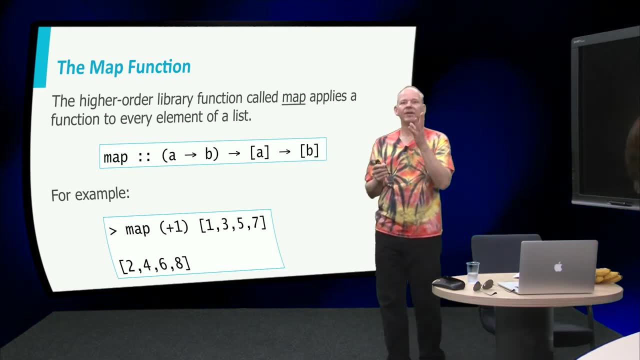 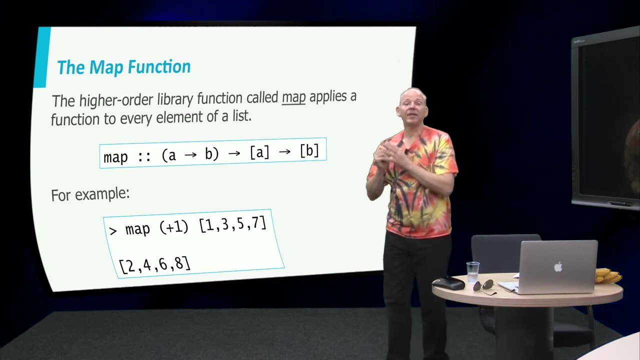 Twice may look like a little weird, it's maybe a little bit syntactic, but here's another higher order function that we use all the time, And this is the map function. So map takes a function and then takes a list and then applies that function to every element of the list. 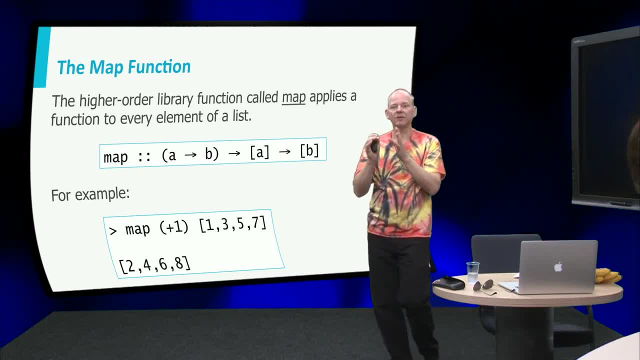 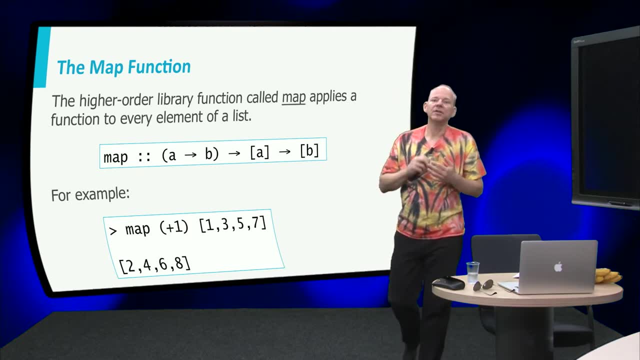 If you look at the type of map, a arrow, b arrow list of a arrow list of b, you have very little choice than to apply that function to every element of the list, Because it kind of you know. 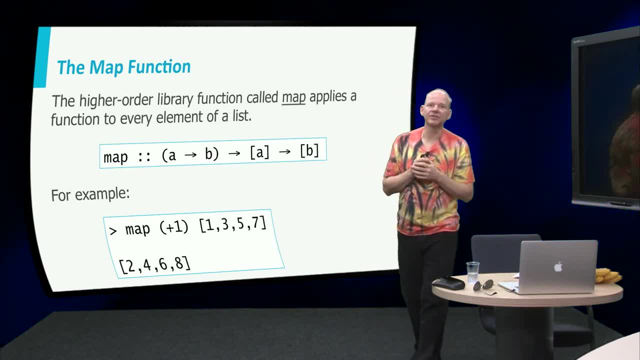 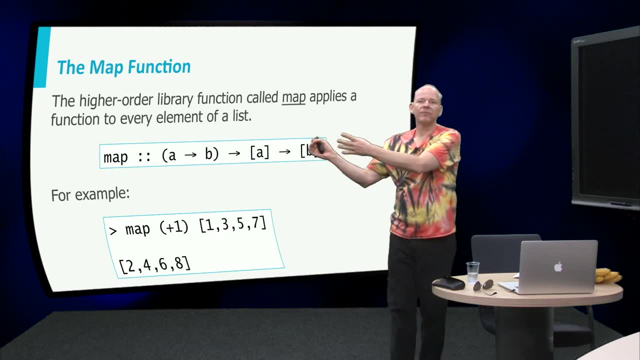 the type really strongly suggests that implementation. You have a function of type a to b. you have a function, a list, with values of type a, and what you require is a list with values of type b. Well, what can you do? 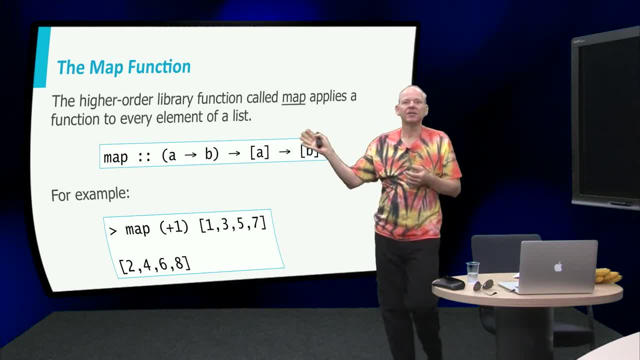 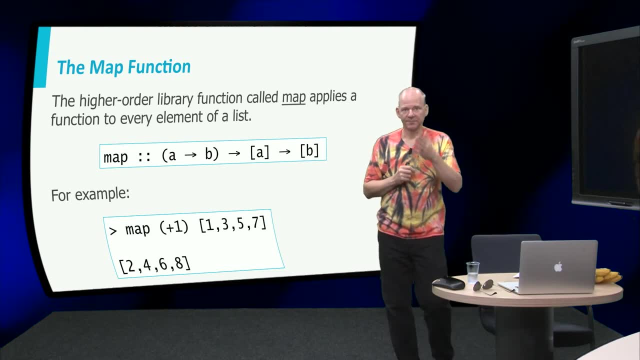 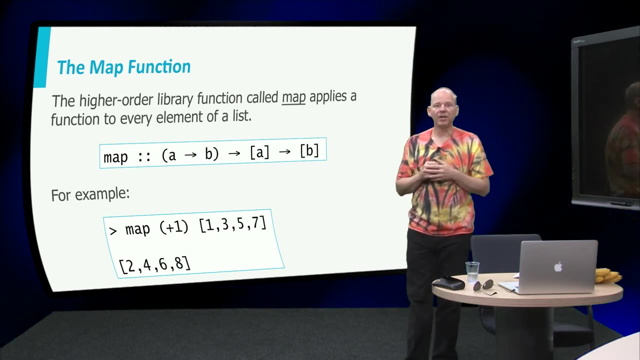 Well, you just transform every element in the input list using that function to get the required output list, And that's exactly how map is defined. Now let's look at an application of map. So we map the sectioned plus function plus one. 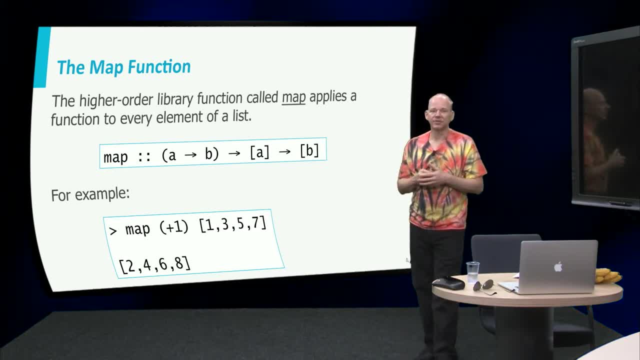 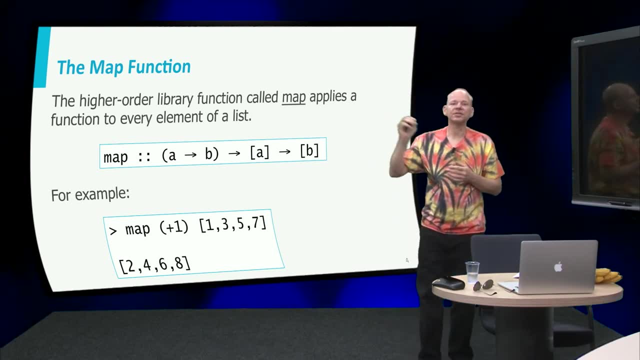 Remember the lecture we had about sections. So this is a function that's implicitly defined to be lambda x, x plus one, And we map that function. we map that function over the list one, three, five, seven. So this function will just add one to every element of the list. 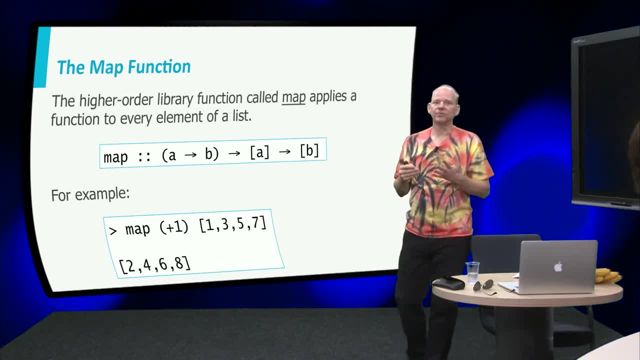 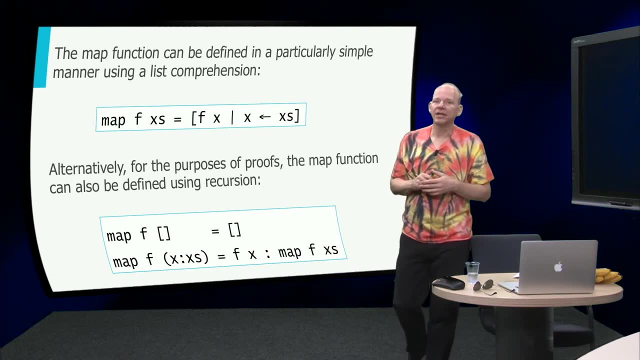 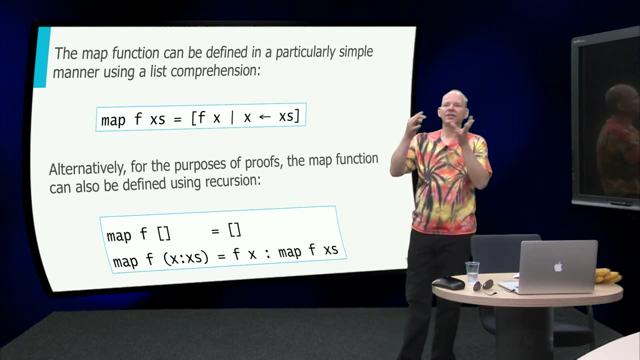 and that's what you see there. We get the result list two, four, six, eight. We can define the map function using list comprehensions very easily. In some sense you can say: list comprehensions are designed to define map, So map applies the function f. 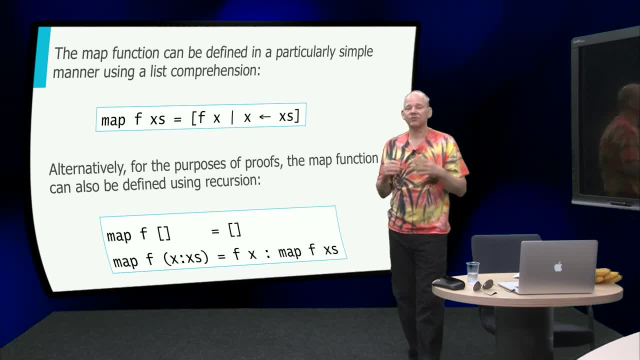 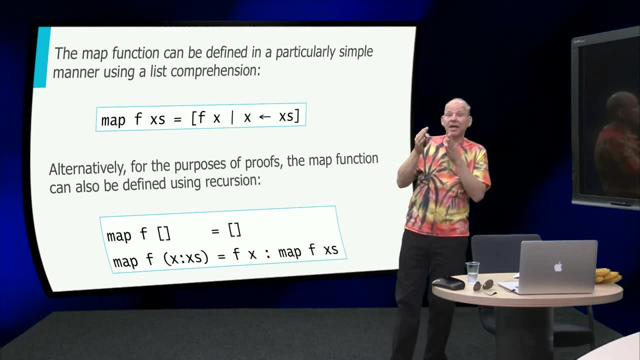 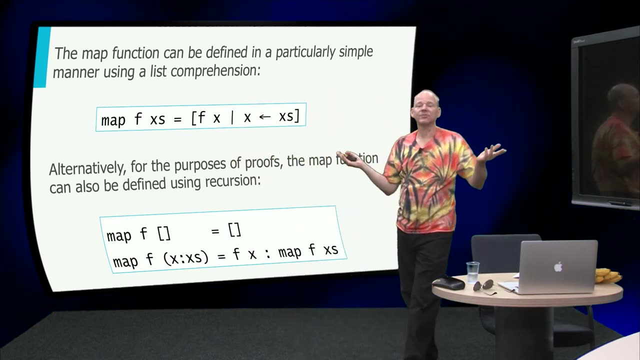 to every element in the list. Now there's the list comprehension. I mean it's like exactly what I said: f. take every element x out of the list axis, apply f to it and return the list. That's what map is. 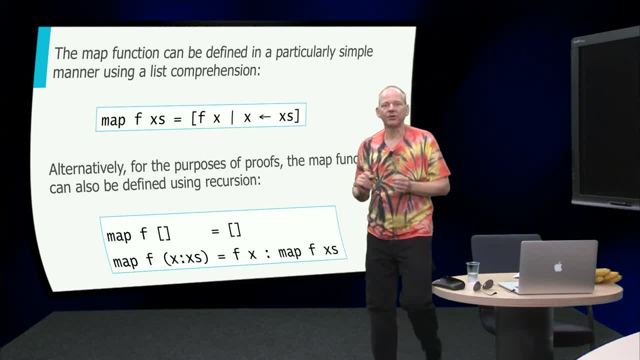 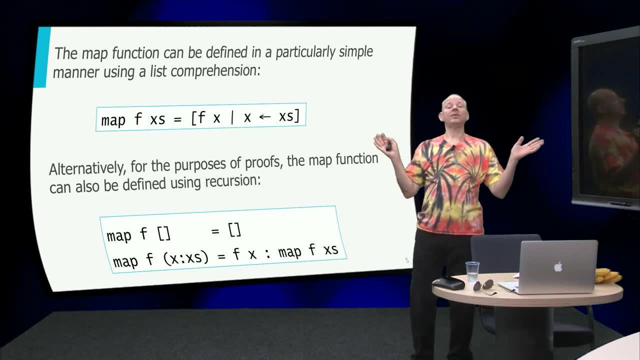 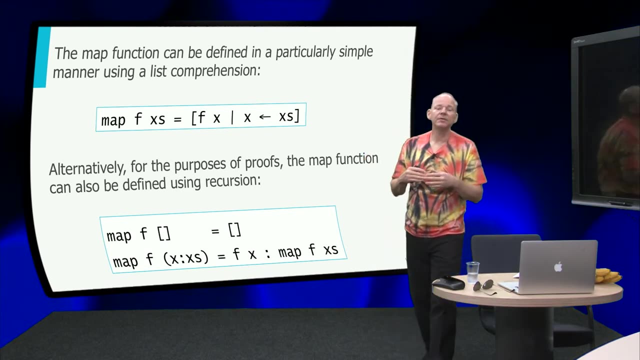 But we can also define map recursively And in some sense I prefer myself the recursive definition. And why do I prefer it And why do I prefer the recursive definition? Well, we will see later that when we define map recursively and we define other higher order functions recursively, 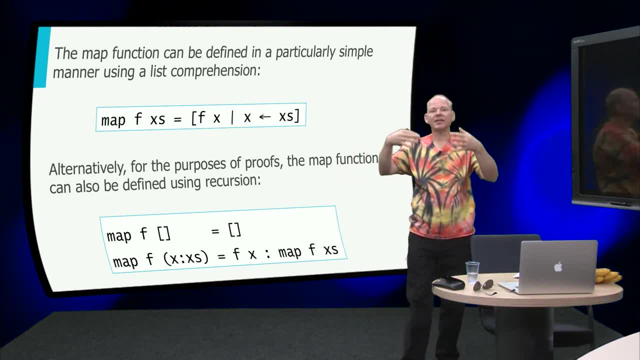 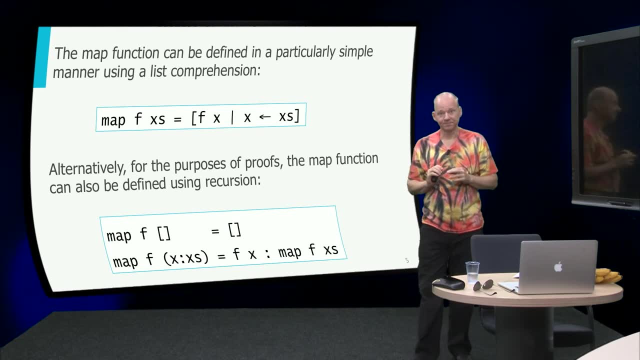 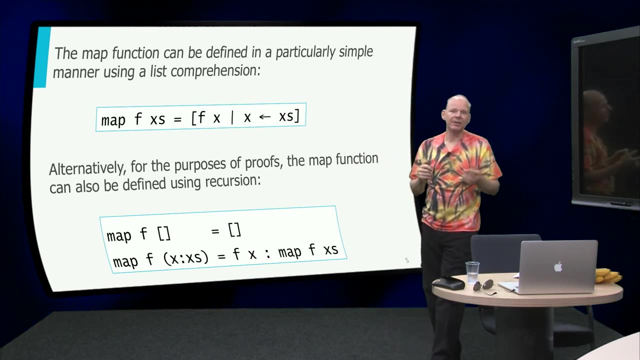 we see a pattern that we can abstract again. So we can abstract map into a super higher order function And that will be the fault function. But for now let's look at the recursive definition of just map. So map of the empty list is the empty list. 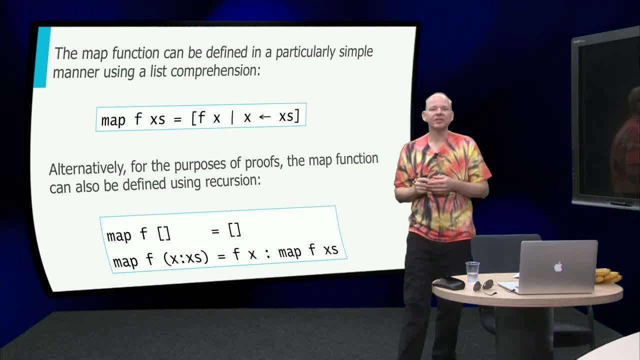 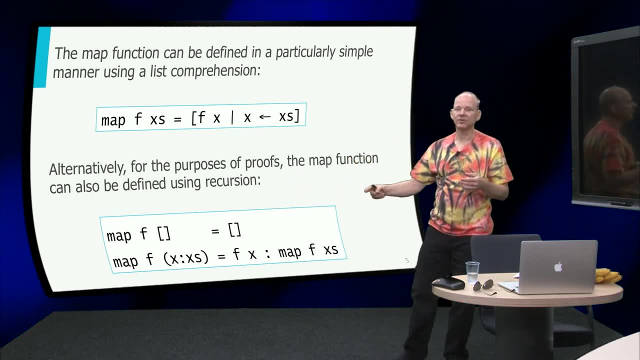 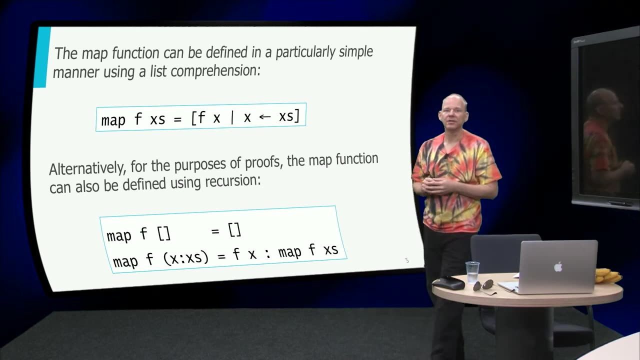 So map of the list: x cons axis. well, what we do is we first recursively map f over axis, So we map f over the rest of the list And then we concatenate f of x to the front. All right, So this is a recursive definition that is inductive over the structure of the list. 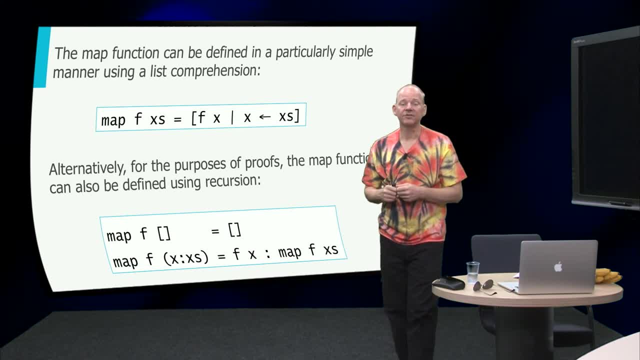 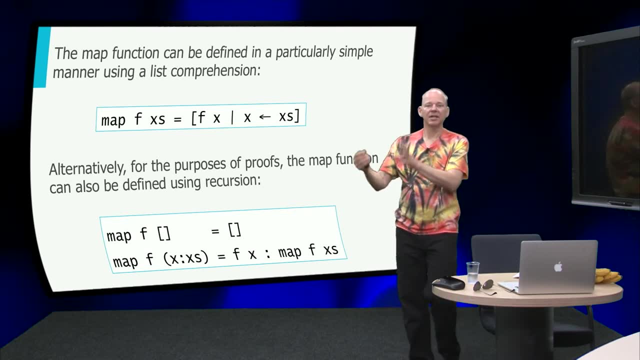 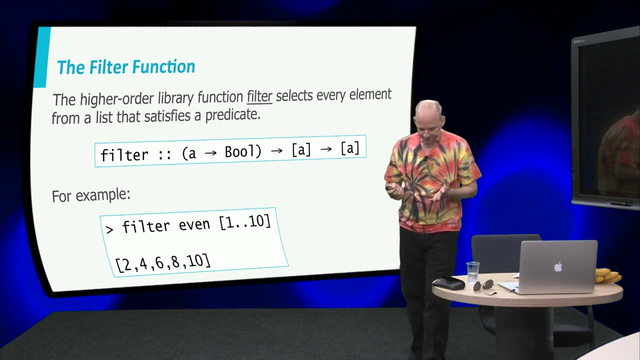 So we have either the empty list or we have the case where the list is built using x cons axis and we recursively map f over the rest of the list and then cons f of x on top. Here's another higher order function, filter. So filter takes a predicate, a function, from a to bool. 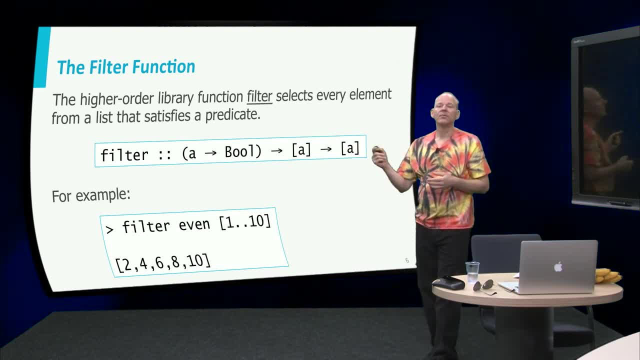 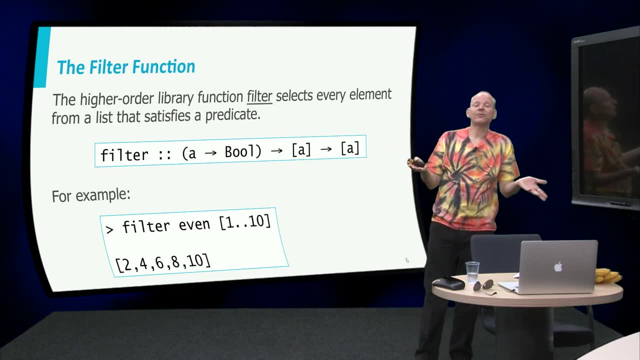 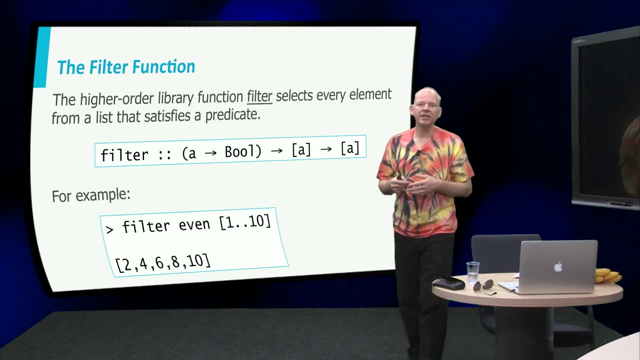 then takes a list and returns another list, a new list, where all the elements for which that predicate does not hold are removed. That's why it's called filter, So all these elements are filtered away. For instance, if we want to filter all the even numbers, 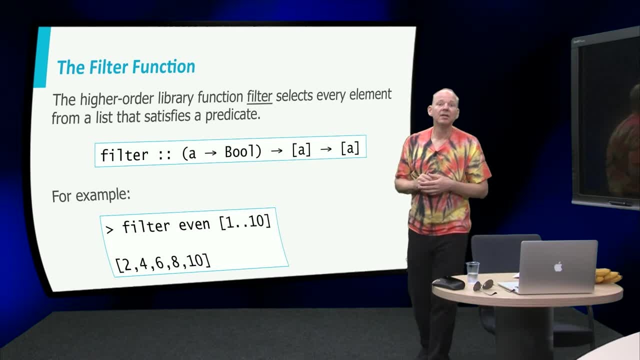 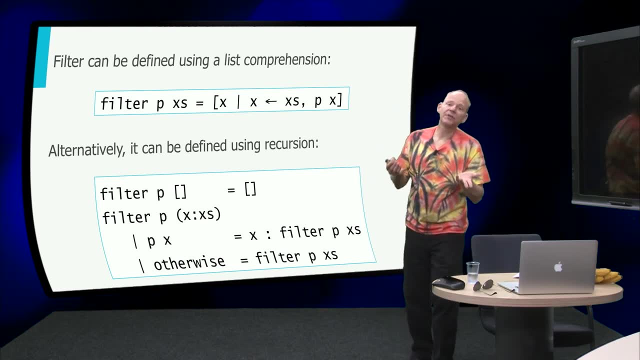 from the list of values from 1 to 10, we get all the even values 2,, 4,, 6,, 8, and 10.. Again, filter can be defined in two ways. First one is with list comprehensions. 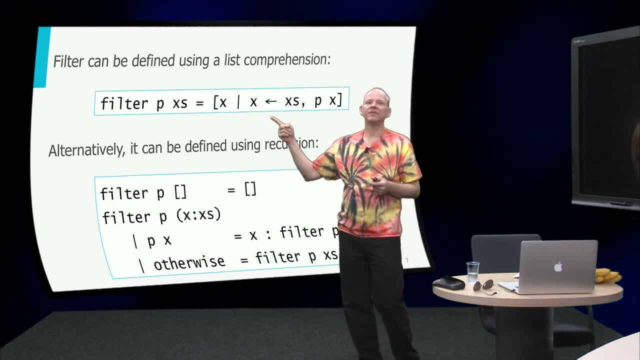 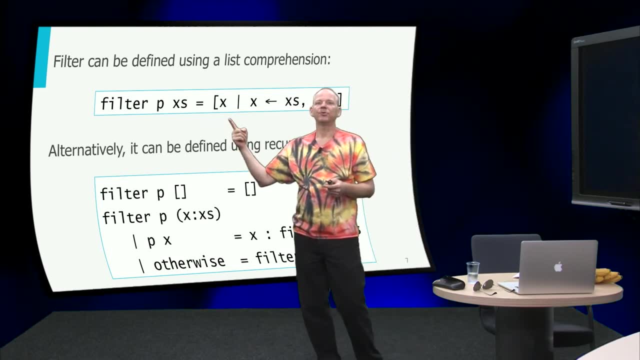 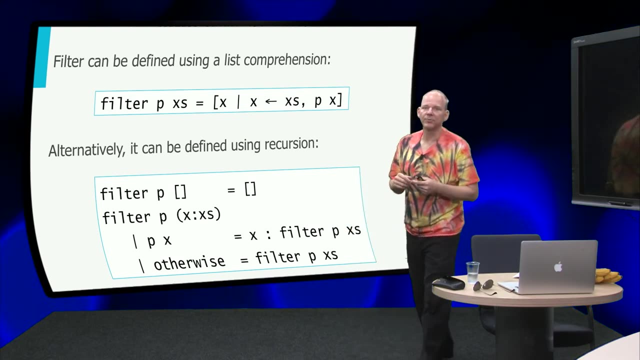 Fairly simple. So what we do is we say: take every element x out of axis, And if p of x is true, then you put x in the result list and that's it. So the definition of filter using list comprehensions looks very simple. 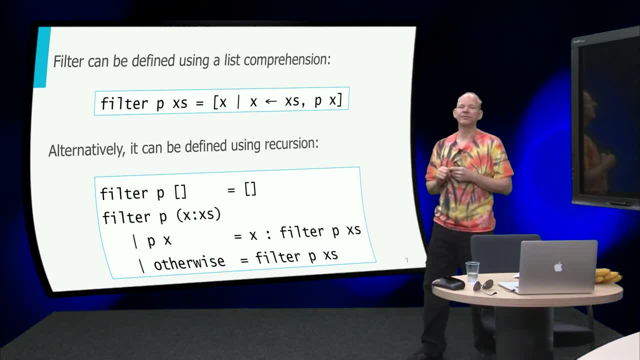 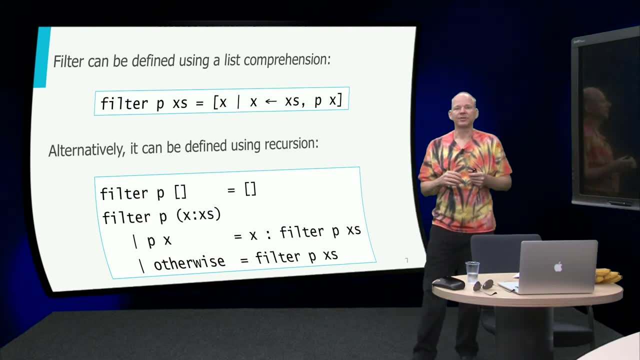 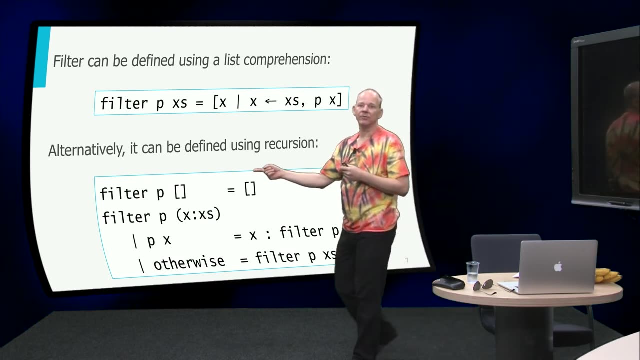 But again, I prefer the recursive definition. And the recursive definition has a very, very similar structure to the map function. It's defined inductively on the structure of the list. So we have two cases: Either we have the empty list. 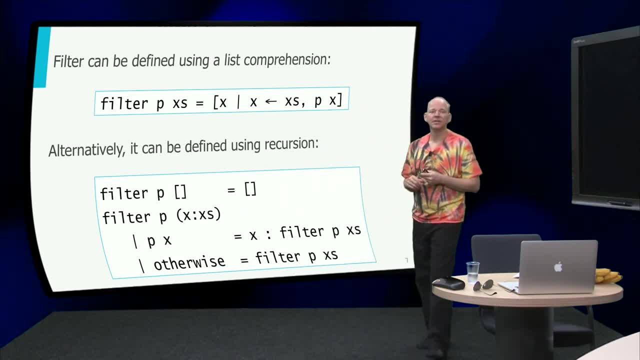 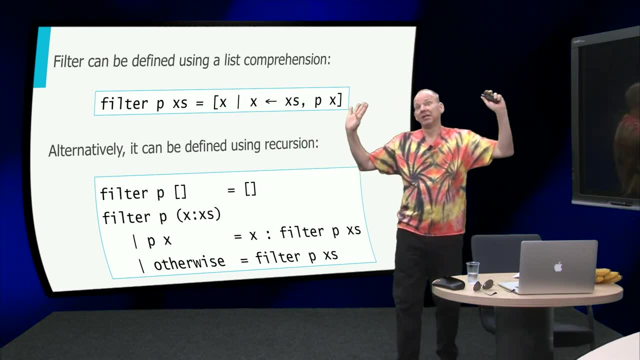 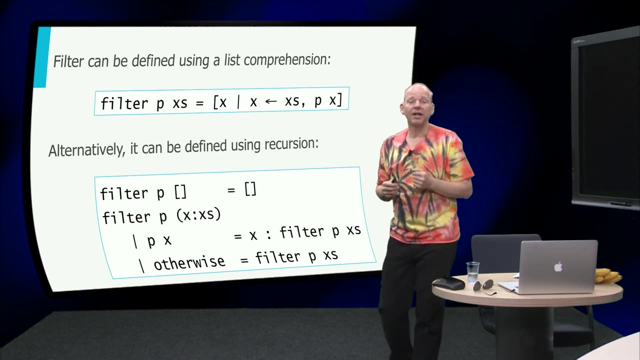 or we have the list x cons x's. When we filter all the values for which this predicate does not hold from the empty list, well, the only thing we can do is return the empty list If we filter out all the values for which p does not hold from the list x cons x's. 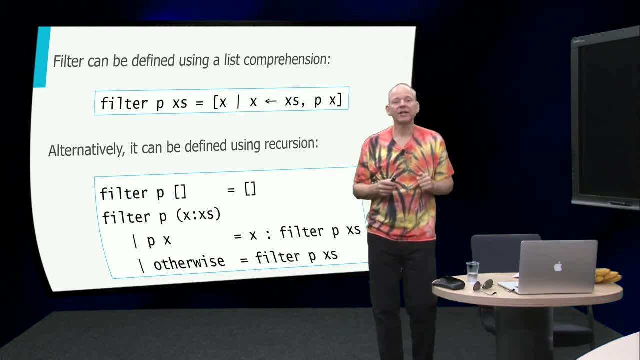 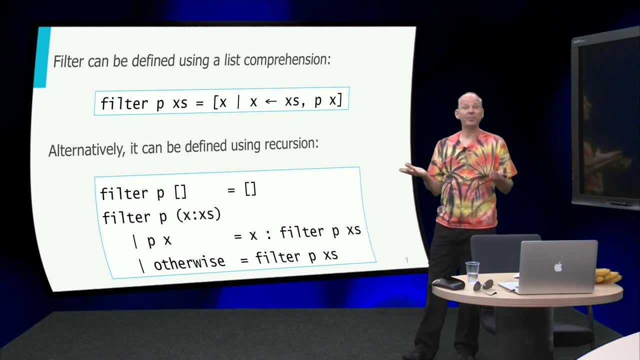 well, there's two cases. First, p of x can be true, So that's this case. This is the second case, when p of x is false. Well, if p of x is true, we filter recursively the rest of the list. 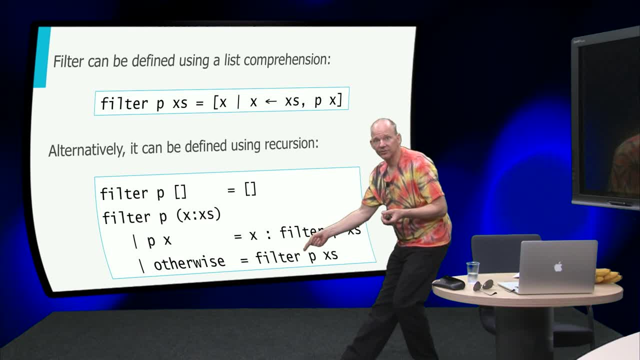 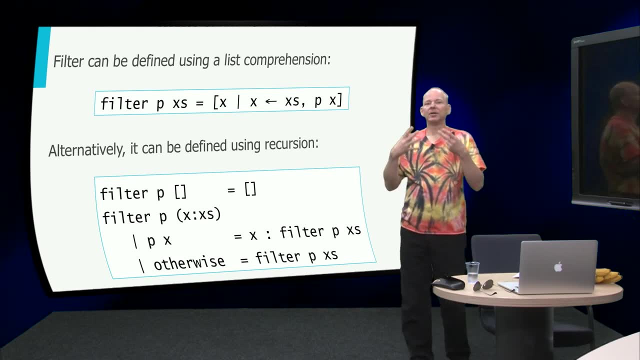 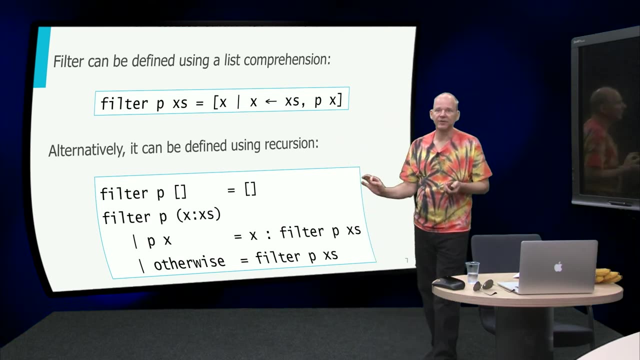 and then we concatenate x on top and otherwise we just forget about x and filter the rest of the list. So here you see, it's kind of as simple as the list comprehension definition. But the important thing is that this definition here follows exactly the same structure of map.